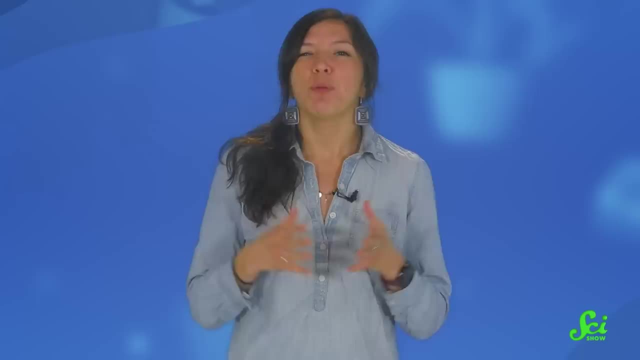 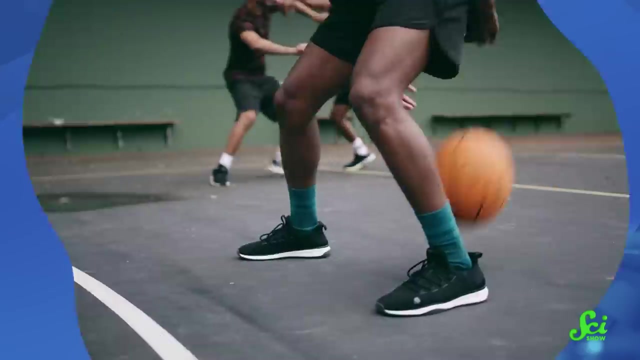 It probably lived in the suburbs and danced to Elvis too. But the 50s weren't just one big uranium party. Every rocket, no matter its appearance, is based on the third law of motion. That's the one that says: if you push something, it pushes back. 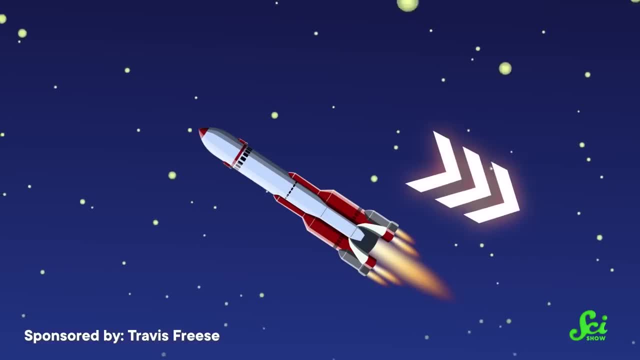 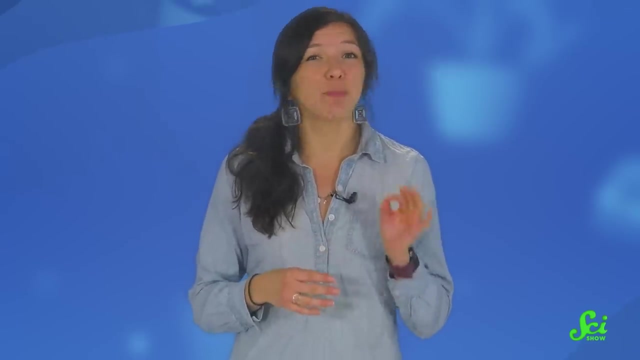 Rockets push exhaust one way, while the exhaust pushes back on the rocket the other way. The harder the rocket pushes the exhaust, the harder the exhaust pushes the rocket. That's rocket science in a nutshell. The hard part is figuring out how to give the exhaust as big of a kick as possible. 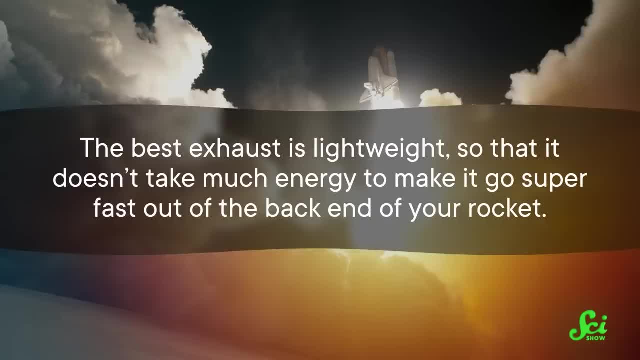 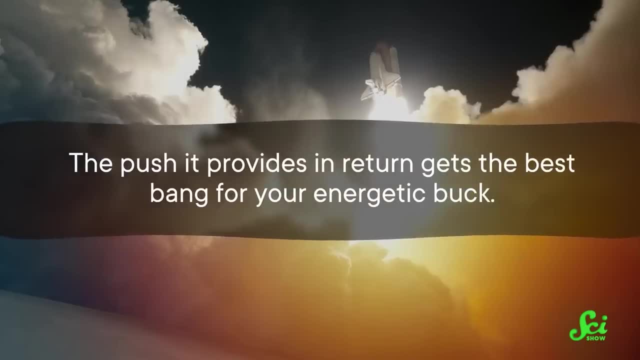 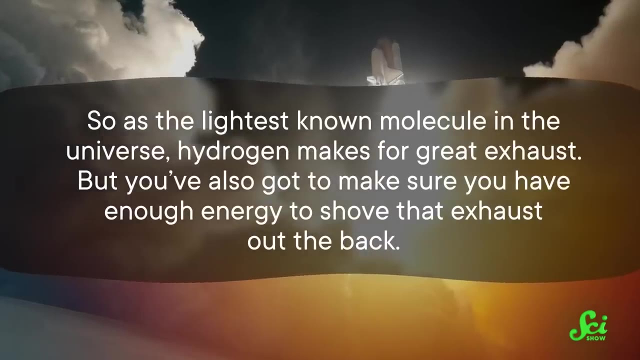 The best exhaust is lightweight, so that it doesn't take much energy to make it go super fast out of the back end of the rocket. The push it provides in return gets the best bang for your energetic buck. So as the lightest known molecule in the universe, hydrogen makes for great exhaust. 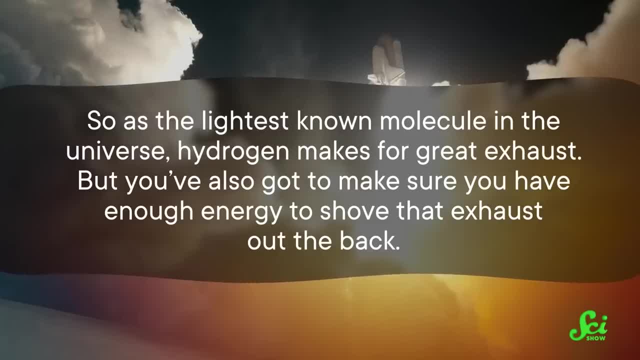 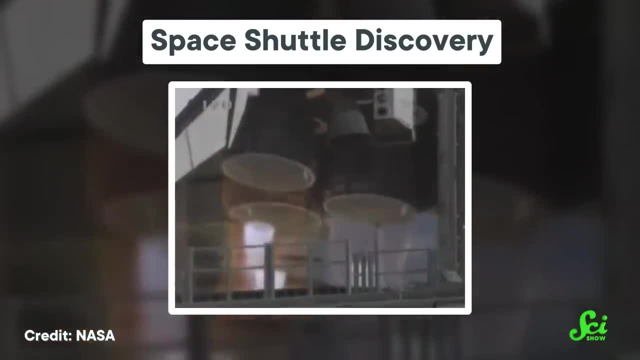 But you've also got to make sure you have enough energy to shove that exhaust out the back. In traditional rockets that energy comes from cracking apart different molecules in your rocket fuel and smushing them back together in new ways. that leaves a bunch of leftover energy. 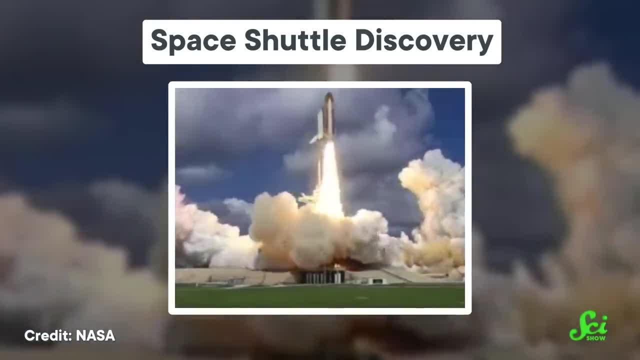 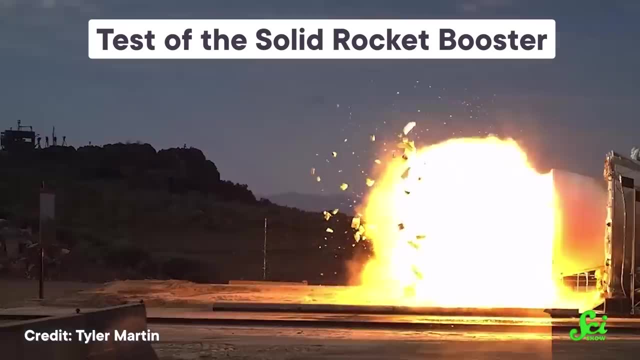 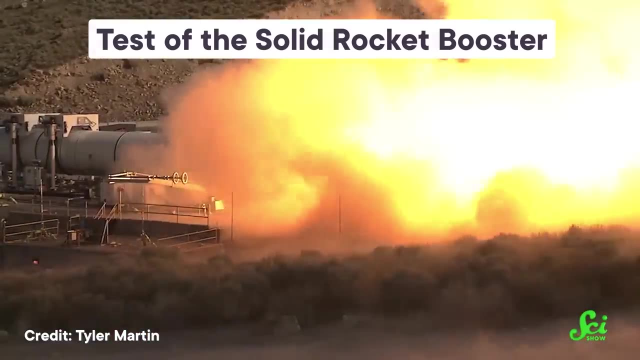 In other words, you're both making the exhaust and the energy to move that exhaust with the same chemical reaction. Hydrogen is pretty awful at releasing extra energy, So instead rocket fuel usually relies on bigger molecules that can release more energy but produce exhaust that's heavier than hydrogen and therefore less efficient in providing. that oomph. Ultimately, in the choice between lots of energy with heavier exhaust or less energy with an ideal exhaust, engineers chose the former. But here's the thing: The laws of physics don't say the exhaust is better than the energy produced by hydrogen. 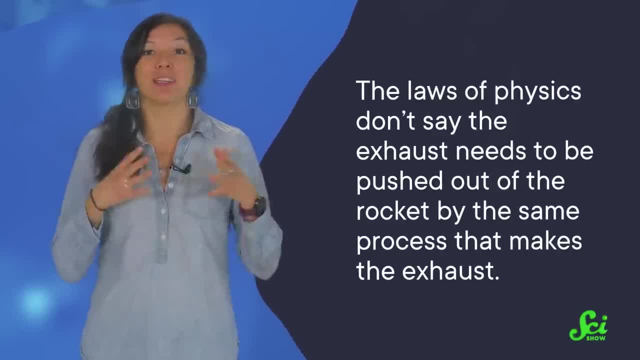 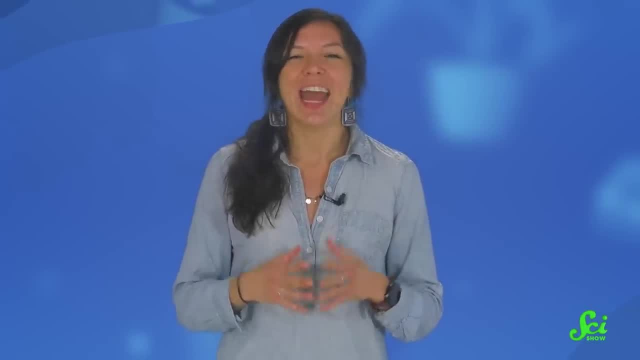 The laws of physics don't say the exhaust is better than the energy produced by hydrogen. The laws of physics don't say the exhaust needs to be pushed out of the rocket by the same process that makes the exhaust. You just need a supply of ready-to-go super-light hydrogen and something that can make a bunch. 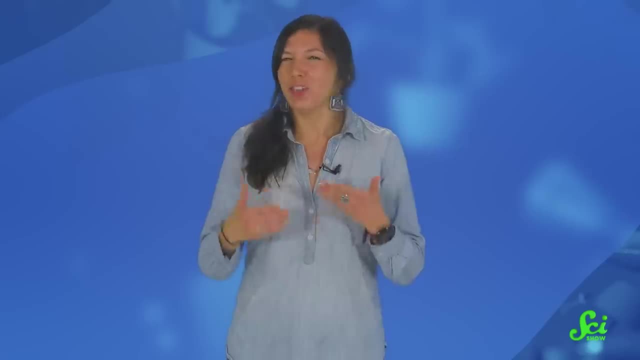 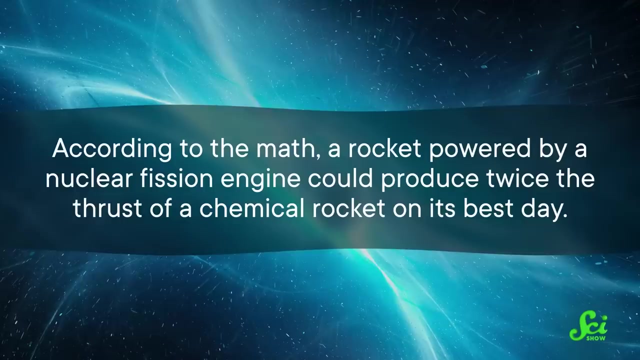 of energy for that hydrogen to absorb. I think you know where I'm going with this. According to the math, a rocket powered by a nuclear fission engine could produce twice the thrust of a chemical rocket on its best day. Plus it would need much less fuel for the same-size trip. The rocket would be both lighter and more powerful than a nuclear fission engine. The rocket would be both lighter and more powerful than a nuclear fission engine And it would be more powerful getting probes or astronauts where they were going a lot faster. So in 1955, not that long after the first nuclear power plant was opened, Project Rover. was born. Research progressed quickly, with successful reactor prototypes starting tests in 1959.. NASA formed around the same time and soon it consolidated Project Rover and other related research under the NERVA banner. Over the years NERVA scientists developed small powerful nuclear reactors that could 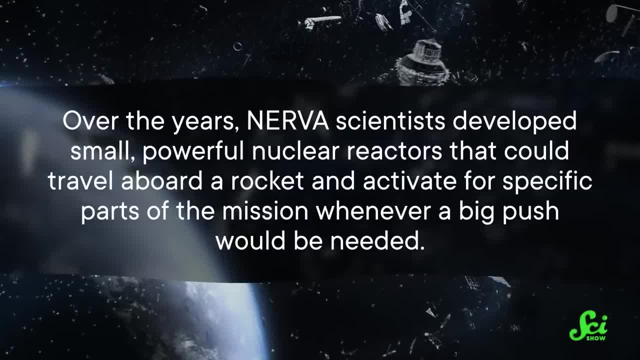 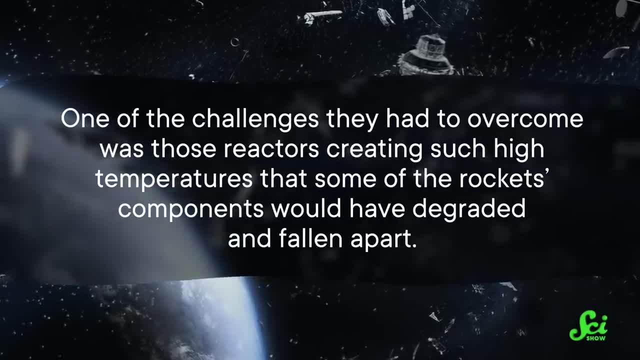 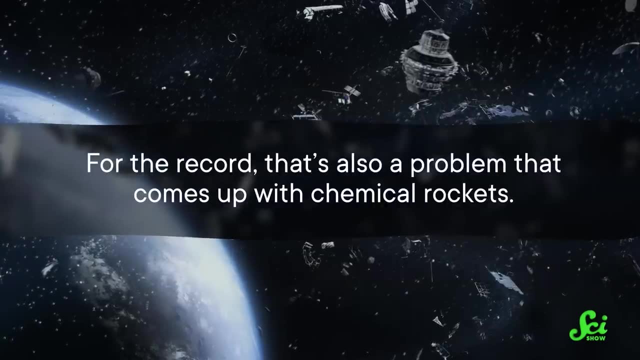 travel aboard a rocket and activate for specific parts of the mission whenever a big push would be needed. One of the challenges they had to overcome was those reactors creating such high temperatures that some of the rocket's components would have degraded and fallen apart For the record. that's also a problem that comes up with chemical rockets. So, as a fix, they designed the engine to circulate some of the super-cold liquid hydrogen through a bunch of tubes to keep everything cool. Hydrogen actually served two jobs. Oh, and don't worry, they also knew they would need to shield whatever cargo or humans. 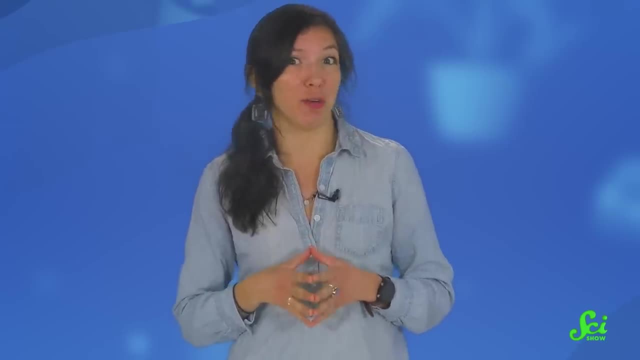 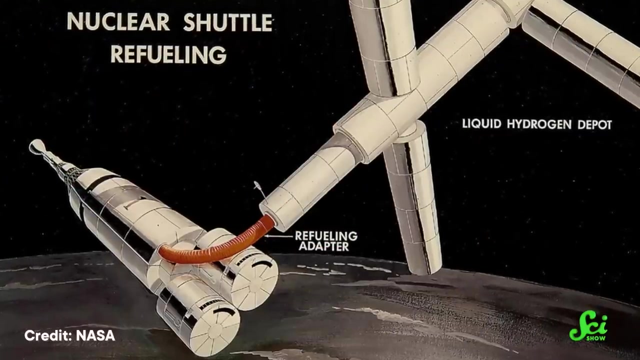 were aboard. They weren't about to risk anyone turning into the Hulk Or just, you know, getting radiation poisoning Soon. people were imagining nuclear-powered shuttles to the Moon or even Mars. The plan still involved chemical rockets for launch, since launches have a high enough. chance of going wrong And you definitely don't want to have to worry about the literal fallout from an active nuclear reactor blowing up a few kilometers above the ground. But once outside the atmosphere the chemical piece would fall away and the nuclear engine would start up. 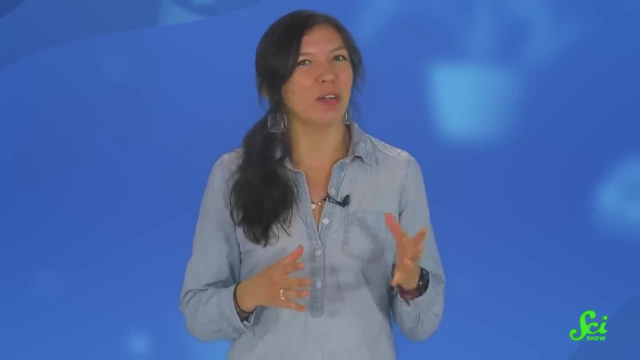 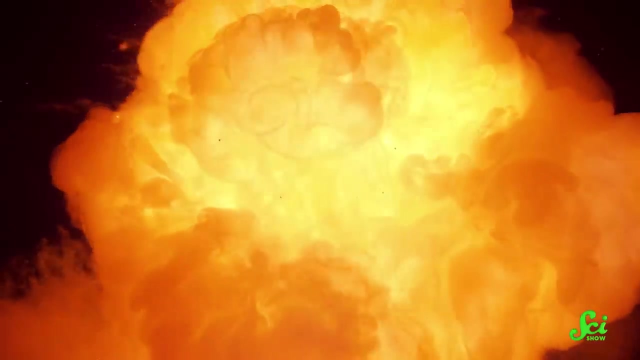 Now, a flying container of uranium is still not ideal, even if the reactors turned off. So in 1965, scientists blew up a model of their reactor with explosives to see how bits and pieces would spread if the worst did happen during launch. 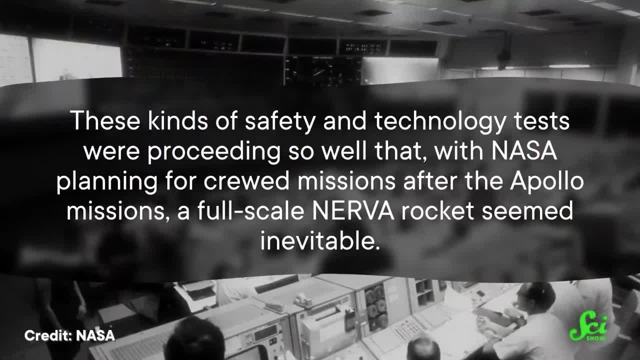 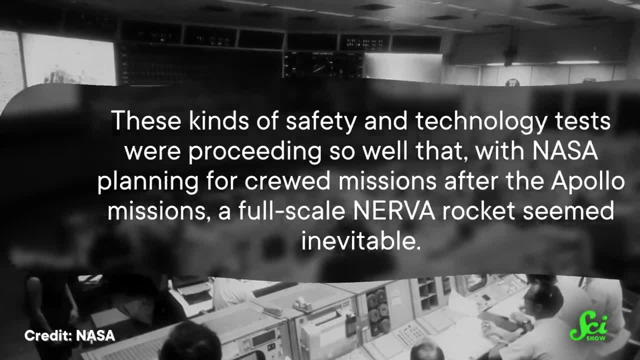 These kinds of safety and technology tests were proceeding so well that, with no evidence, NASA was planning for crewed missions. after the Apollo missions, a full-scale NERVA rocket seemed inevitable, But NASA's budget was shrinking even before astronauts reached the Moon. 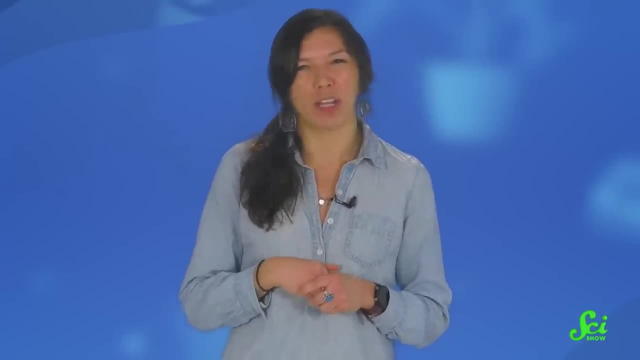 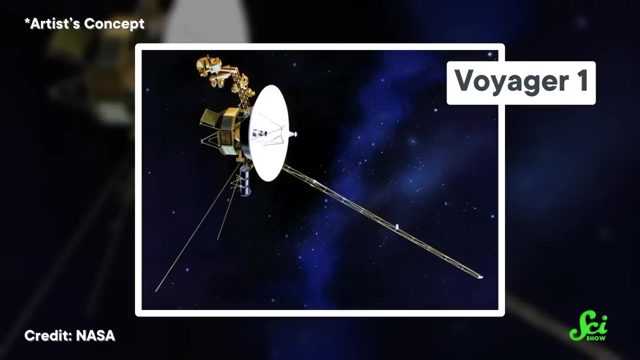 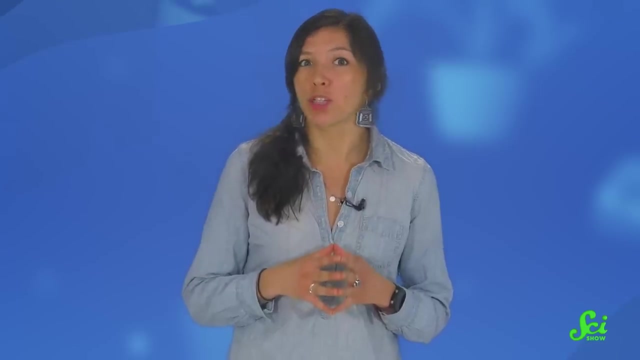 Long-term, long-distance human spaceflight wasn't a priority. By 1973, NASA had to choose between NERVA and what would become the Voyager missions. They chose the Voyager, Which honestly not a bad choice. Every 10 years or so, though, scientists glanced back at nuclear-powered propulsion with flurries. of interest in the mid-80s, the early 90s and the mid-2000s. But even as satellites have employed all sorts of other non-chemical thrusters over the last few decades, nuclear rocket engines still haven't reached space. 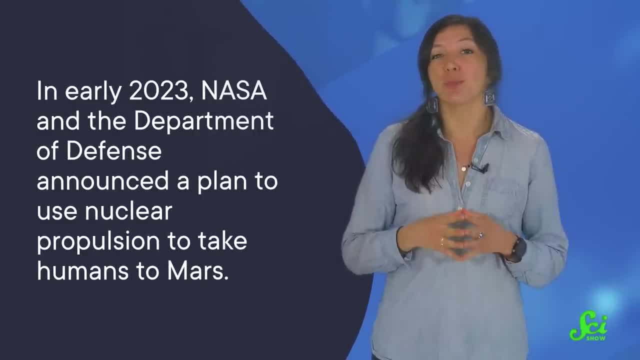 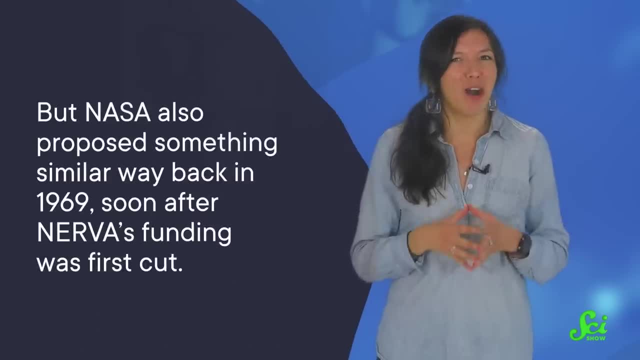 At least not yet. In early 2023,, NASA and the Department of Defense announced a plan to use nuclear propulsion to take humans to Mars, Which is awesome. But NASA also proposed something similar way back in 1969, soon after NASA's launch of. 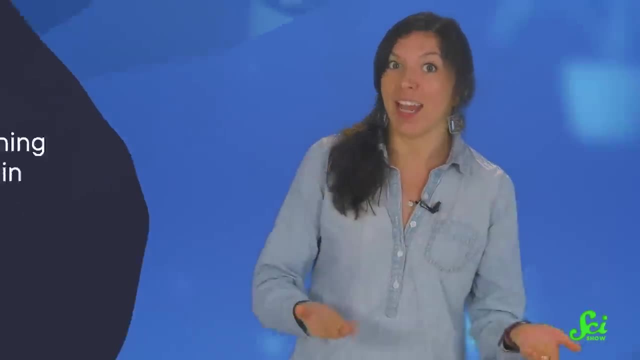 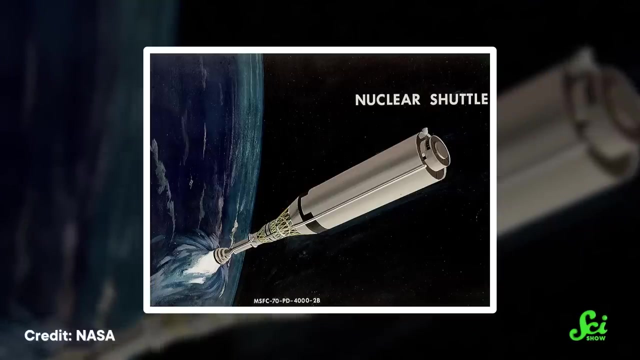 the NERVA rocket. The project and NERVA's funding was first cut And then again in 1991.. So for now, nuclear-powered propulsion remains a well-verified laboratory curiosity. But soon, maybe, it will have its day in the Sun.